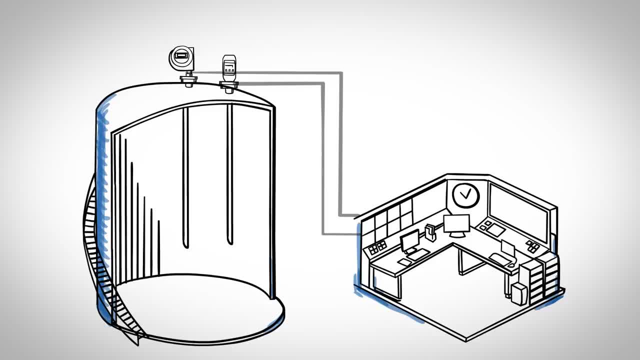 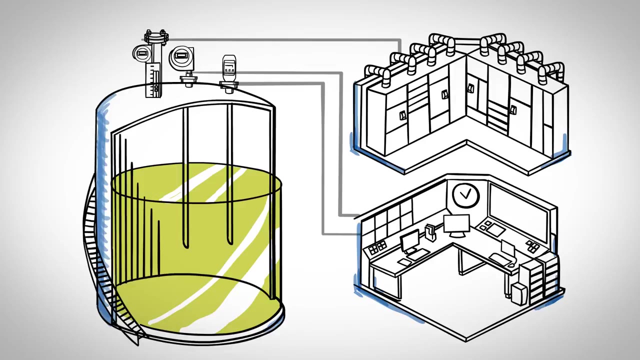 back to the control room. The level indicators trigger a high-level alarm if the tank reaches a specified level. Tanks also have an independent high-high-level alarm set to sound when the product reaches an even higher level in the tank. High-high-level alarms are powered from the motor control center on a separate electrical circuit, independent of the primary level indicators. 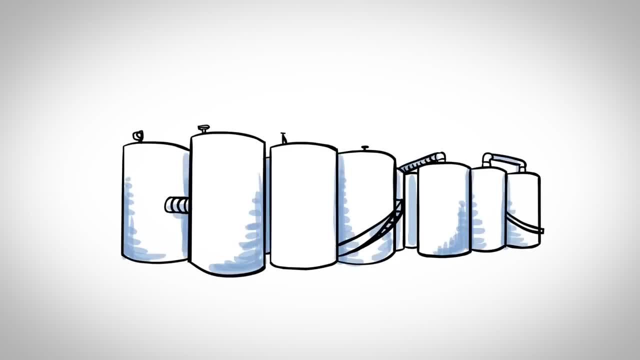 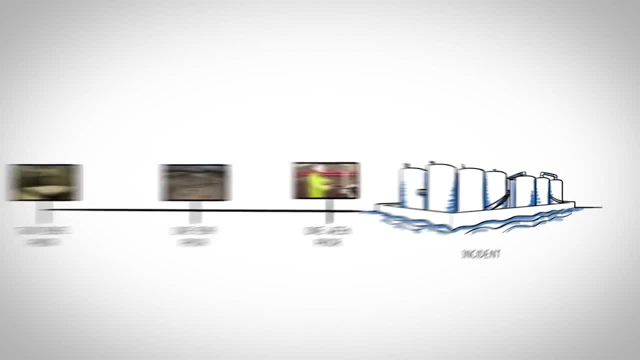 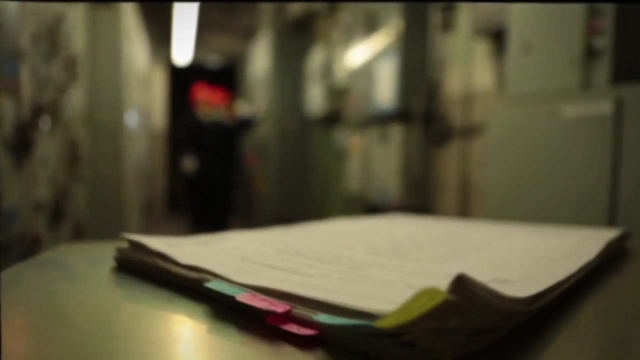 Additional safeguards to reduce the potential consequences of a tank overfill are provided by a berm surrounding the tank farm and by emergency shutdown systems at the refinery Two years prior to the overflow. the electrical distribution system was modified as part of a plant upgrade. 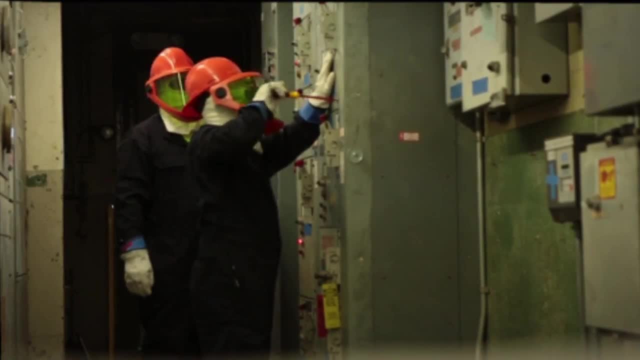 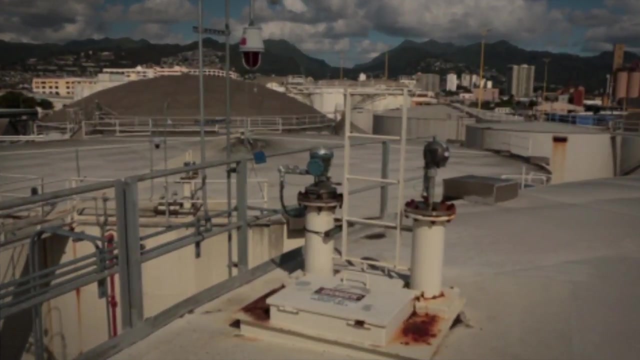 Power circuits for the primary level indicators were moved from main breaker 15 to breaker 21.. The systems were tested and power loads validated. However, the electrical drawings were never updated. One year prior to the tank overflow, the high-high-level alarm on the tank was replaced and the same model was ordered for the replacement. 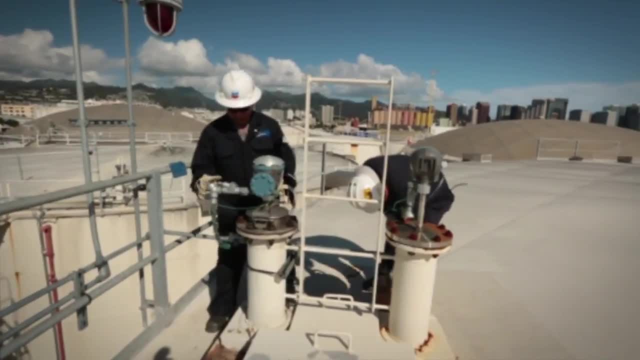 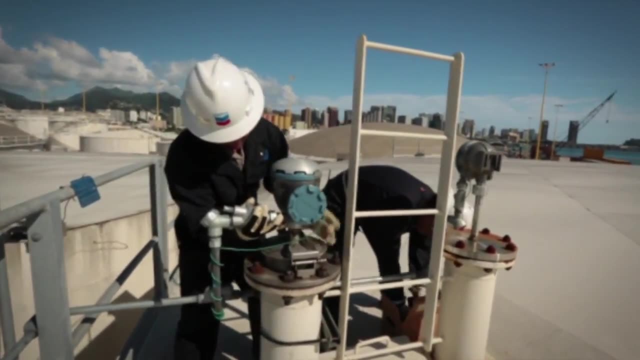 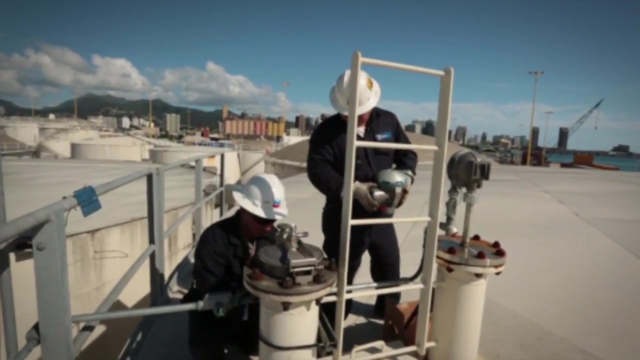 After receiving the new high-high-level alarm, maintenance installed it believing it was a replacement in kind. However, the device was actually an upgraded model that required different scaling and calibration than the original unit. As a result, the high-high-level alarm was not properly transmitting tank level to the control room. 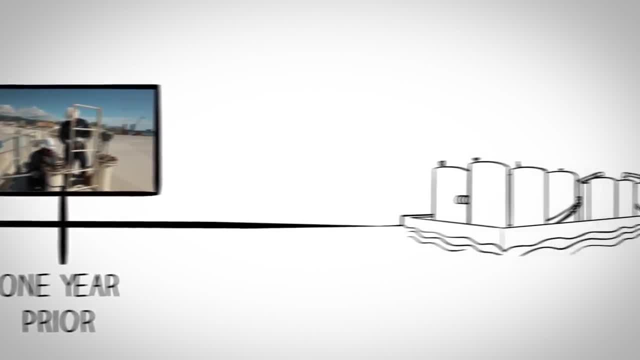 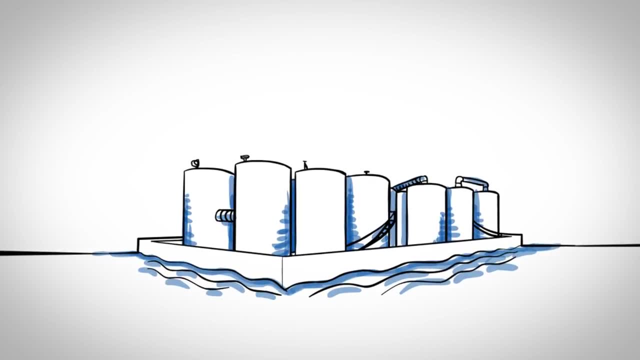 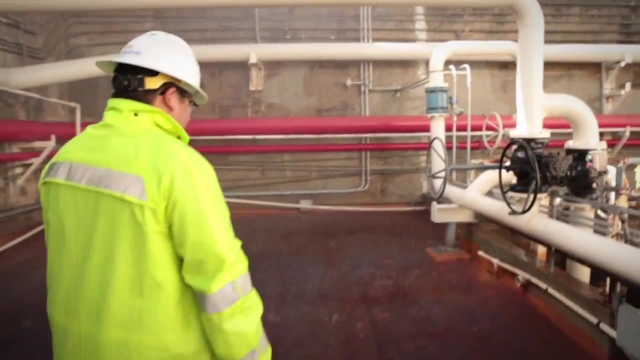 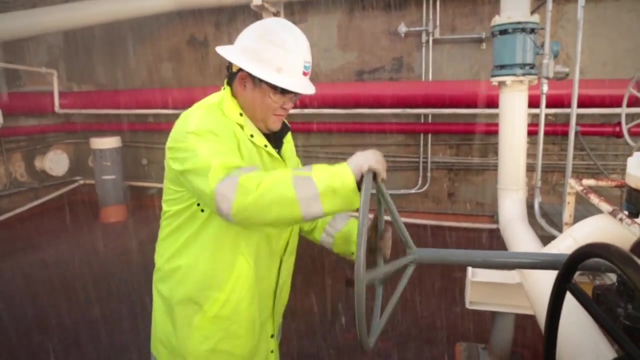 The mistake was not recognized when the device was received and installed and went undetected during periodic testing programs. A week prior to the incident, the area experienced two days of heavy rainfall and water began collecting inside the berm. In accordance with procedures, the water was verified to be free of contaminants and the drain valves were opened to allow the clean rainwater to drain to the ocean. 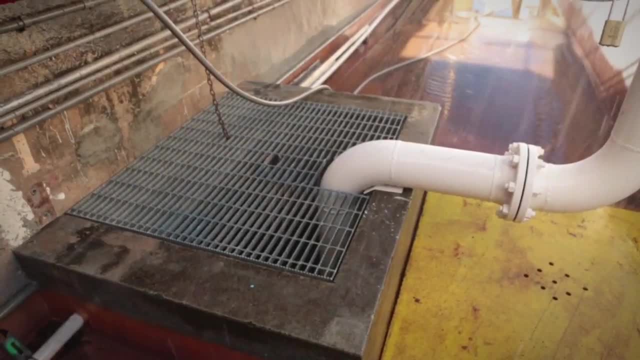 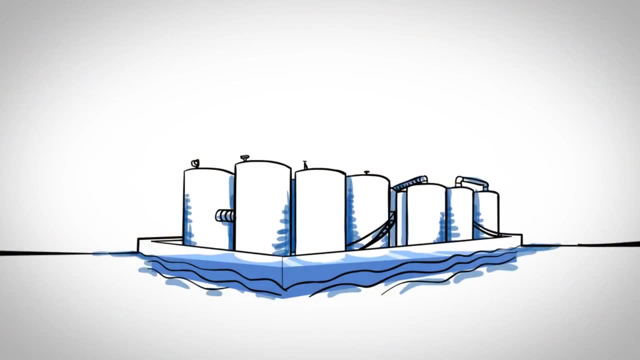 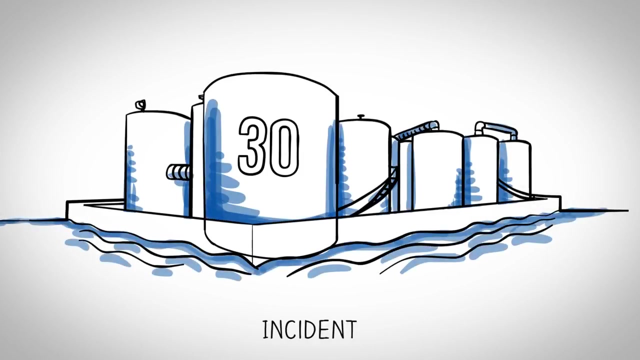 But after opening the drain valve, the operator was called away to another task and neglected to note the open valve on the checklist for shift change turnover. As a result, the drain valve was left open On the day of the incident. Tank 30 is receiving gasoline by pipeline from the refinery. 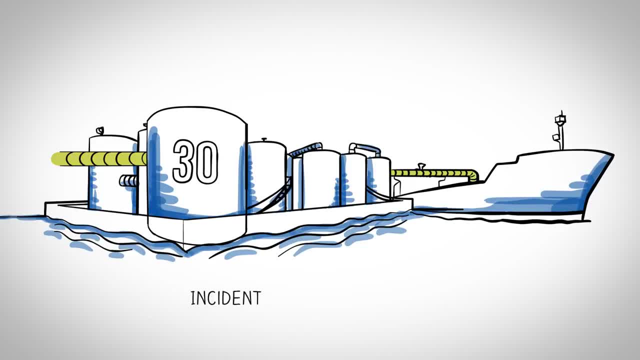 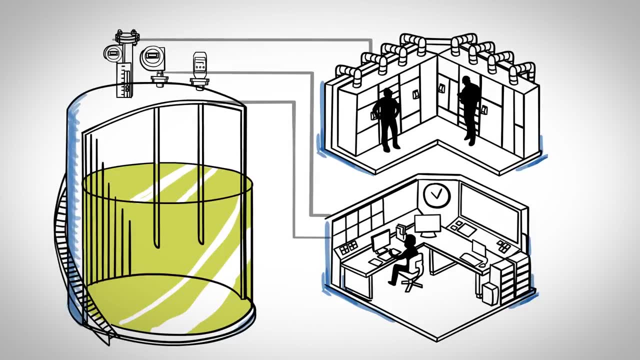 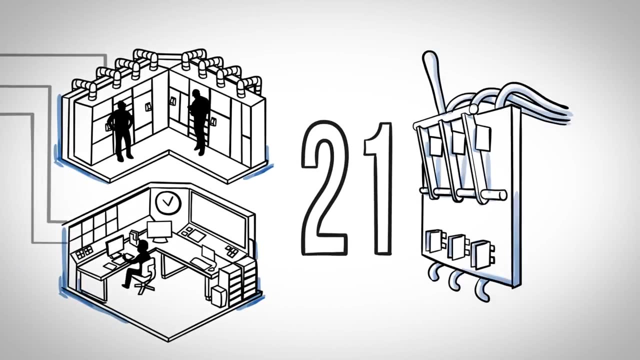 Simultaneously, Jet A fuel is being offloaded to the Hilo Bay export tanker. Operations are running smoothly. Meanwhile, an electrical crew is preparing to perform maintenance at the facility's main motor control center. Work was permitted to isolate Main Breaker 21 from service prior to performing the maintenance tasks.